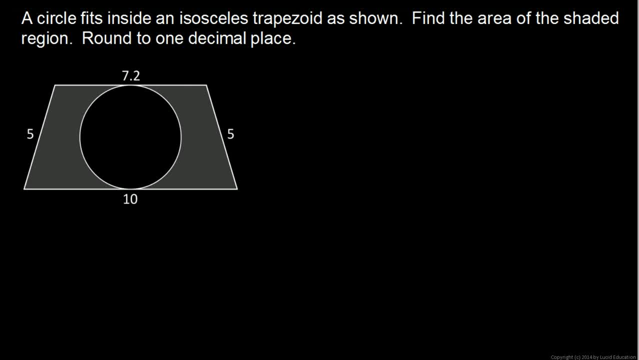 the average of the two bases times the height and we need to draw in the height and the height is going to be perpendicular to the bases. So draw that in. We'll call it h. Go ahead and draw it in on both sides. That's h in both places. 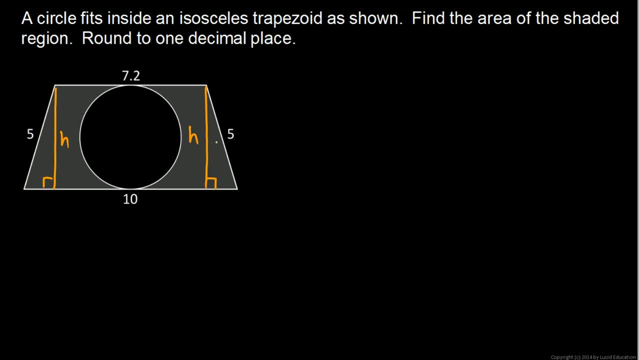 Now notice that this forms two little right triangles, one on each side and this bottom edge. let's give it a name. We'll call it x, and that will be the same on both sides. Now we can find x pretty easily. Okay, look at this. This is length 10, all the way across. 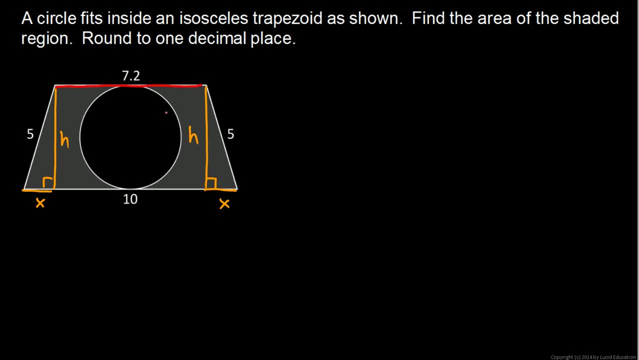 and look at this 7.2.. If this is 7.2 up here, then we're going to have a length of 10.2.. So we're going to have a length of 10.2.. Then, from this point across to this point, that will be 7.2 also. So this means 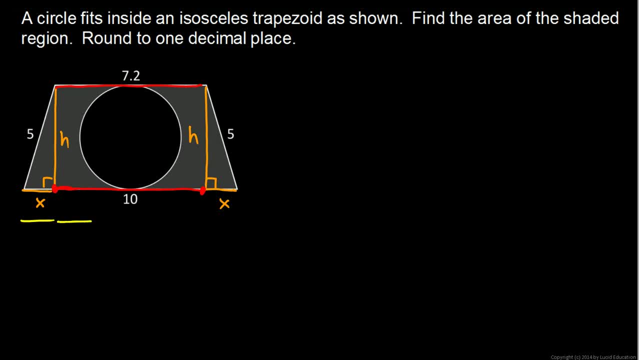 that x plus 7.2 plus x has to add up to 10.. So let's write that. I'll write it like this: 2x plus 7.2 equals 10, and then we'll do a little bit of algebra: Subtract 7.2 from each side. 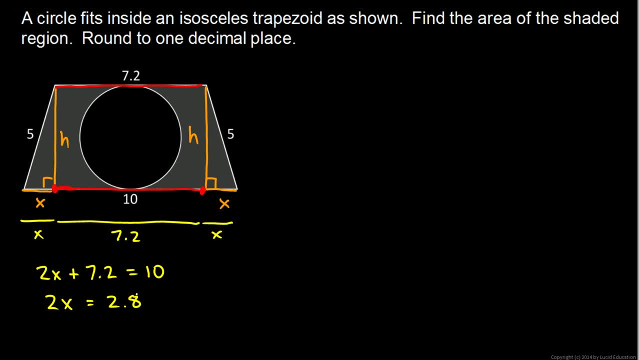 and you get: 2x is equal to 2.8.. So x is equal to 1.4.. Then we can take one of these small triangles and apply the Pythagorean theorem. I can write: h squared plus 1.4 squared is equal to 5 squared, So h squared- just rearranging this, will be 5. 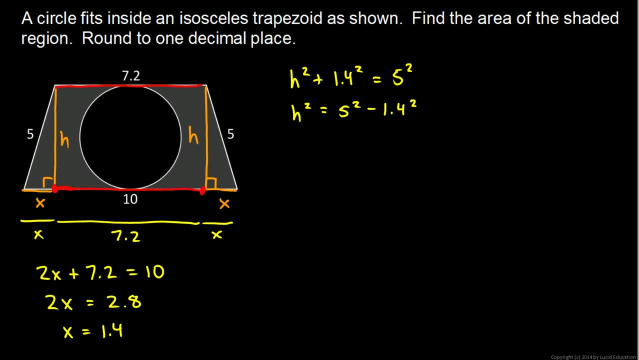 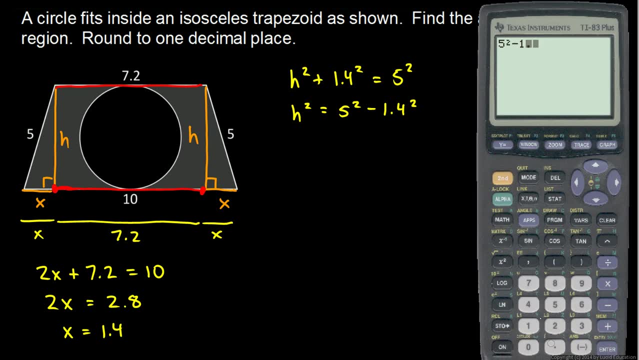 squared minus 1.4 squared. So h squared plus 1.4 squared is equal to 5 squared So h squared, and we can figure that out. Let's pull up the calculator: 5 squared minus 1.4 squared is 23.04.. 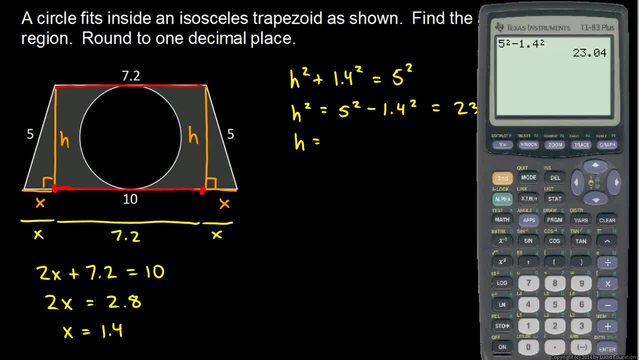 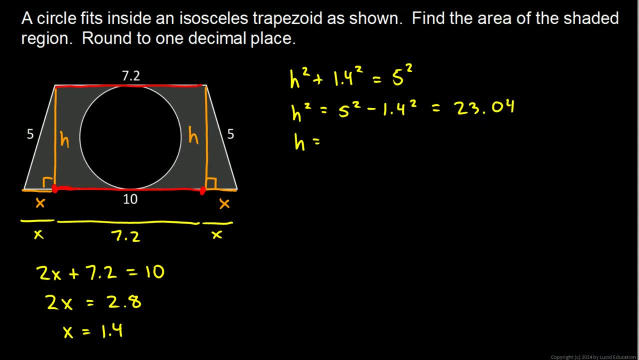 So h will be the square root of that. So the square root of 23.04 is 4.8.. So the height is 4.8.. That's my height, h. Now I can find the area of the trapezoid. That's the area of the trapezoid and that will be the 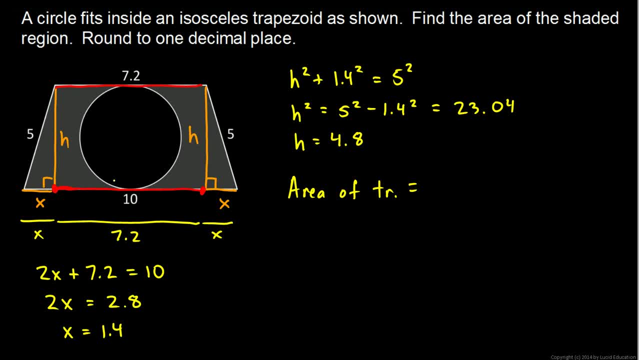 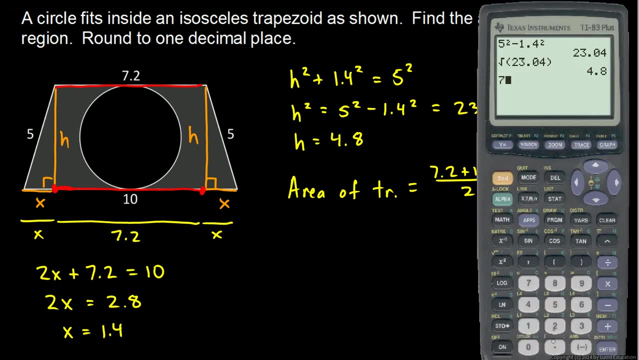 average of the bases. So that's 7.2 plus 10 divided by 2 times the height, and the height is 4.8.. And so we work that out: 7.2 plus 10 divided by 2 times 4.8.. I got 41.28 for the area of the trapezoid. 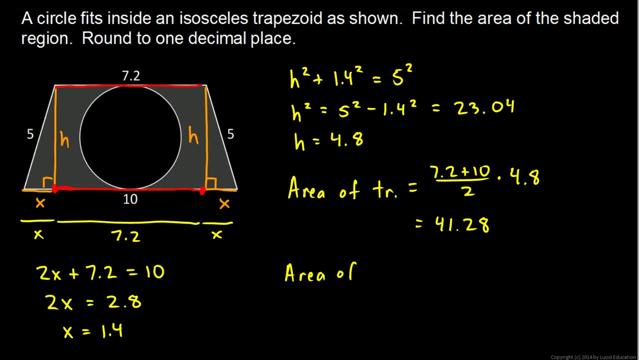 And then the area of the circle- area of a circle is just pi? r squared. Okay, Now let's take a look at the area of the trapezoid. Let's take a look at the area of the trapezoid. 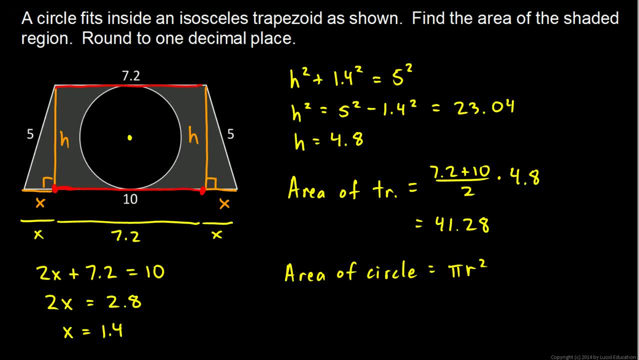 How do we find the radius here? Let's draw it in the center to one edge. If you look at the diagram, you can see that the radius here will be half the height, And that's pretty easy. You can do this in your head. 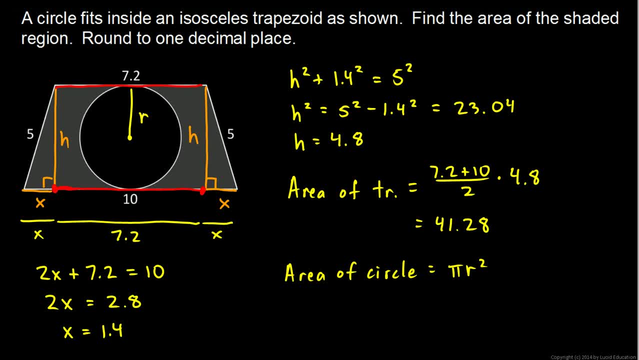 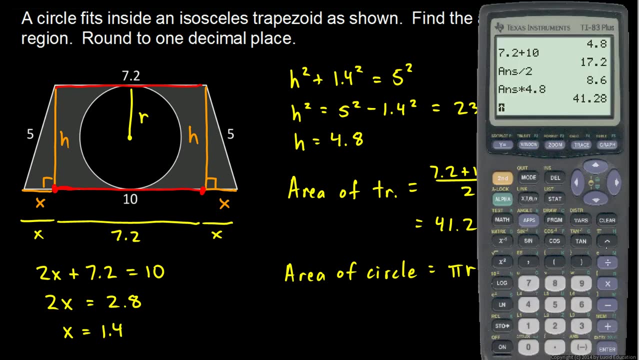 The height is 4.8, so the radius is 2.4.. So the area of the circle will be pi times that radius, 2.4 squared. So let's calculate that Pi times 2.4 squared. Pi times 2.4 squared comes out to 18.. 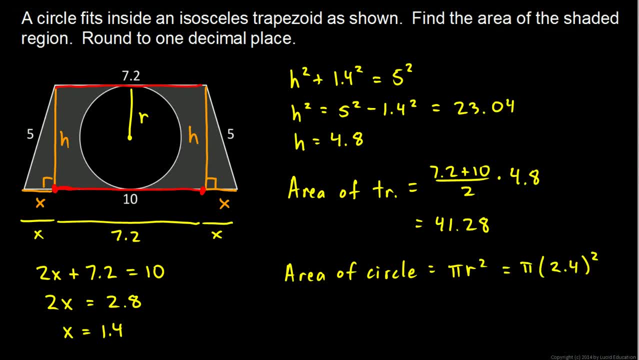 I'll round that to 18.1.. So the area of the circle is equal to 18.1.. And so then the area of the shaded region will be the area of the trapezoid. That's 41.28 minus the area of the trapezoid.